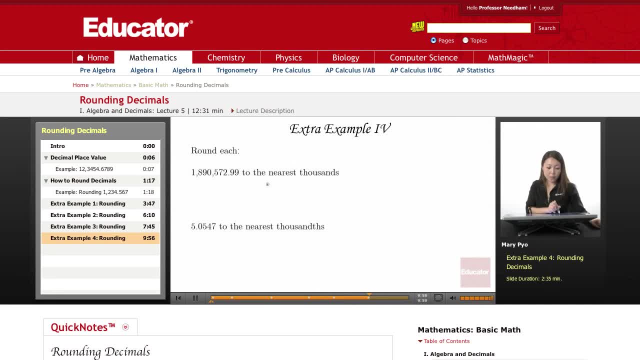 Okay, this number to the nearest thousands, No th. That means the thousands is the number right before the first comma, right? So right in front of the first comma is a thousands. So I'm going to circle that. The number before it is a five, It's five or greater. So that means I have to change this zero to a one. 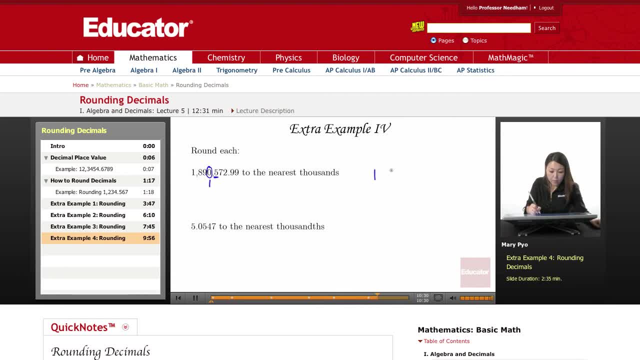 So I'm going to write all the numbers before it. So one, eight, nine, And instead of writing the zero, I'm going to write the one. Okay, write my commas And then remember, all the numbers after the circled number are going to turn into zeros. So this was my circle number, right? That changed to one, zero to one, So it's going to become zero, zero, zero. 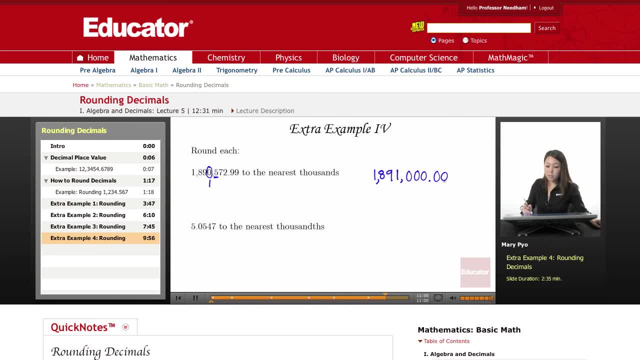 Point zero, zero. And again, because these zeros are at the end of a number and they're behind the decimal point, I don't have to write them out, Okay, but I could. if I want, I can just leave it like that. Okay, So this is the number when you round this to the nearest thousands. Now, this one is to the nearest thousandths with the th. Okay, so that means it's, we know it's behind the decimal point. Here's tenth. 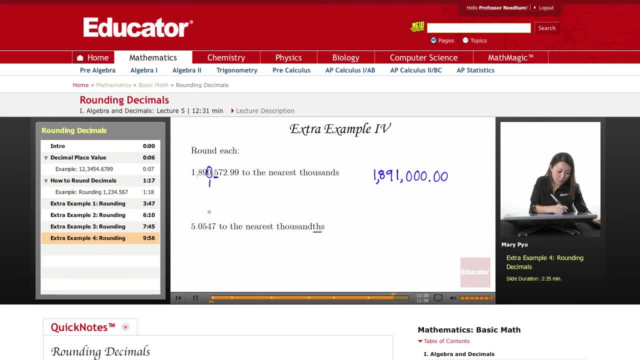 hundredths, thousandths. Okay, so then I'm going to round to that number. I circle it, look at the number behind it. it's a seven. It's five or greater, right, Seven is bigger than five. That means I change the circled number to a five. I round up. Okay, so again the circled number. it's either going to stay the same, if this number behind it is smaller than five, or it's going to become one bigger.